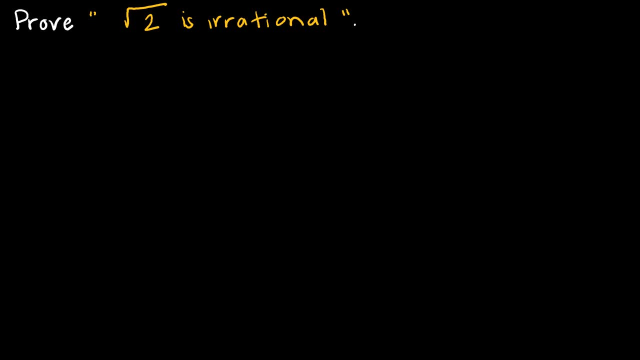 by contradiction. and what that means is we start by assuming: suppose, radical 2 is not irrational, or of course it makes more sense to say is rational, We're going to assume that not P is true And this is not P. So what do we know about rational numbers? Well, we can then say: then 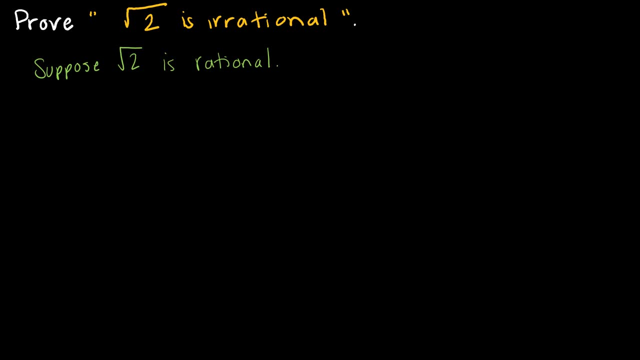 radical 2, oops, let's start again. then there exists two integers, a and b, such that radical 2 equals a over b. So where did that come from? Well, that is, the definition of a rational number is that it can be written as a ratio of two integers. I also must conclude that 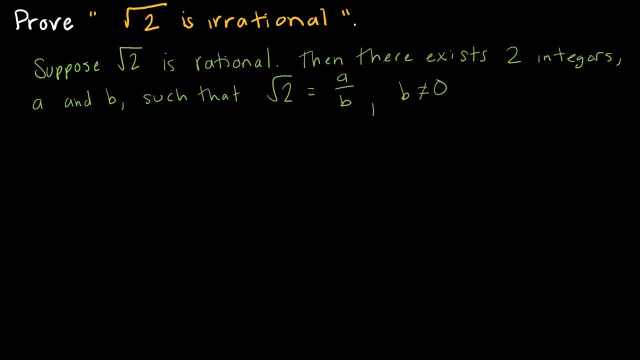 b cannot be 0 because of course, we cannot divide by 0. and- and this is I'm just going to give to you, but this is something in chapter 4 we'll discuss, And this is something we'll discuss in chapter 4.. And a and b have no common factors. 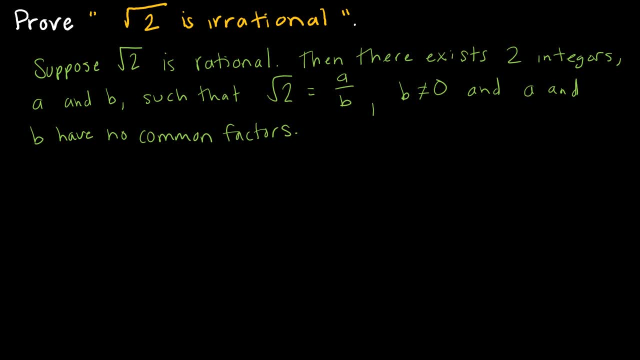 So that is all of our assumption. Now, in a proof by contradiction, we're going to start proving essentially what we're trying to prove, which is that radical 2 is rational, and we're going to keep going until we reach a contradiction that says: oh wait that. 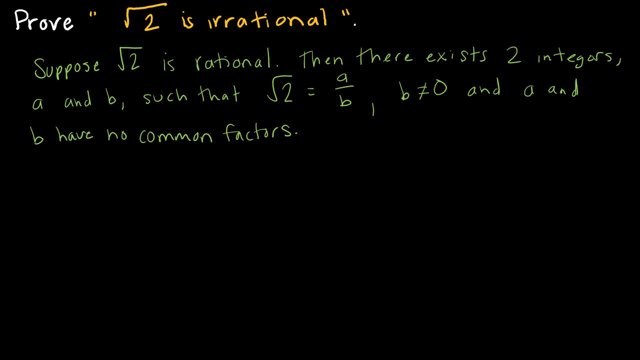 couldn't have been the case. So we're going to keep going until we reach a contradiction that says: oh wait, that couldn't have been the case because it interferes or contradicts something that we assumed at the beginning of the question. So, without further ado, we've got radical. 2 equals a over b. 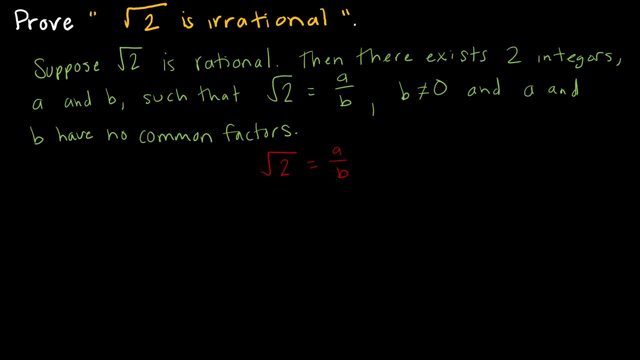 because I said so? because that is what a rational number is. Let's say, I square each side, that gives me 2 equals a squared over b squared. So far, so good. Then I can say: well, that means 2b squared is equal to a squared, just by multiplying. 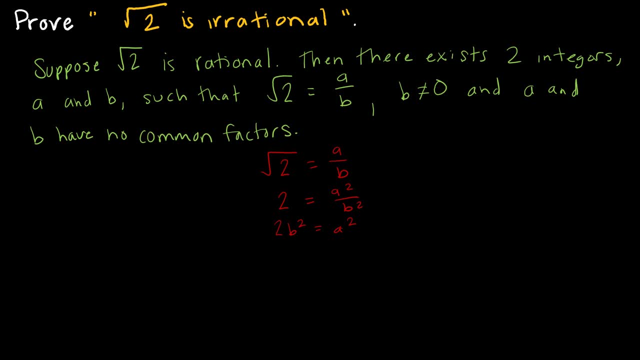 each side by b squared. Now what does this tell me? This tells me that a, squared, must be even. Excuse me, that a must be even because we know if we square an odd number, we get an odd number. So this tells me that a must be even. So, since a is even, I can say that a equals to c for some integer c. 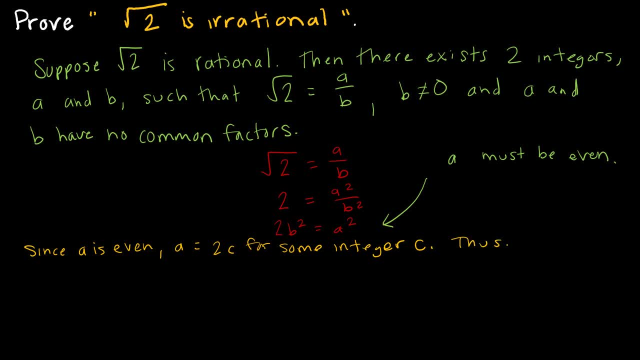 Thus- now I'm going to do some more math- I can say 2b squared equals 2c squared and 2b squared equals 4c squared, because I've squared it, and therefore b squared is equal to 2c squared. 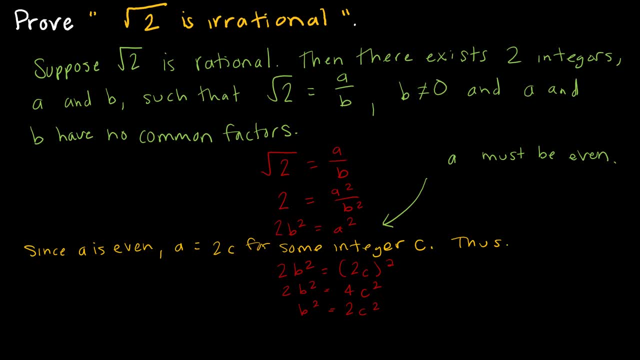 Well now, where does that get me? Well, this tells me that b must be even Because of this 2, just like here, because of this 2.. Now, why is this a proof by contradiction? At the beginning of this I said a and b have no common factors, but we know that if a is even and b is even, 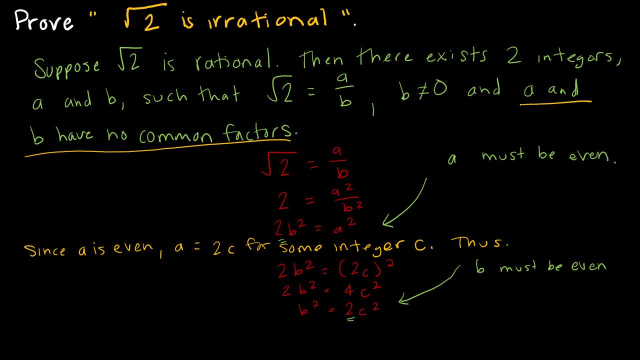 therefore, they do have a common factor. So we have found a fact that contradicts one of our original assumptions. So we have found a fact that contradicts one of our original assumptions. So we have found a fact that contradicts one of our original assumptions. 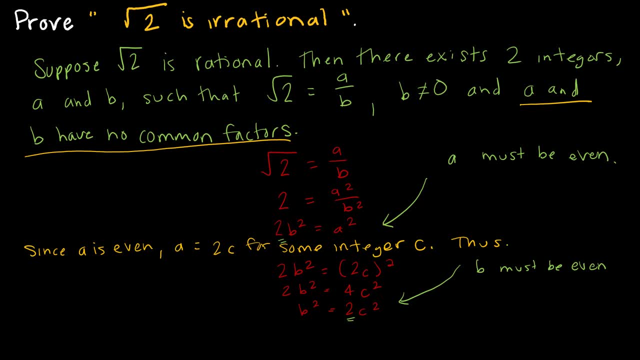 So we can say. So we can say- Oops, lost my pen- Since a and b have a common factor, Since a and b have a common factor, Since a and b have a common factor, This contradicts our original assumption. 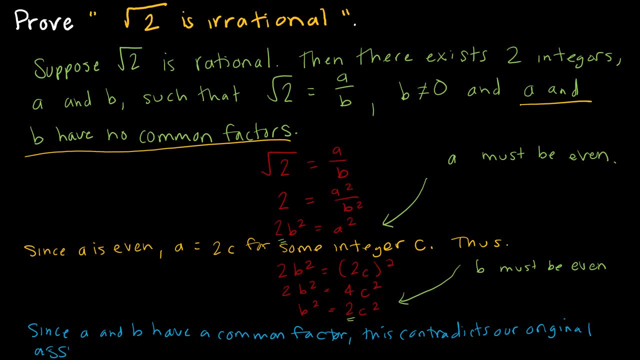 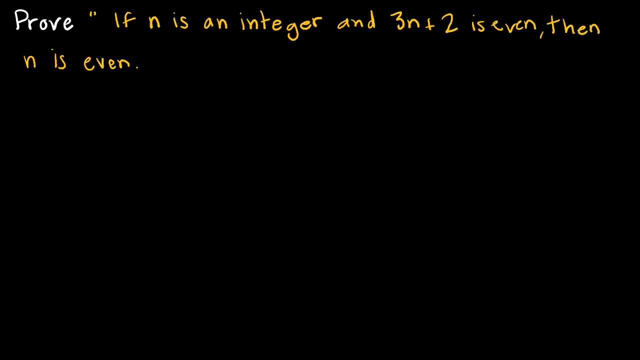 This contradicts our original assumption, And we're done, So here's another for us to try together, and hopefully this one looks familiar to you. We've actually already proved this using contraposition, and now we're going to try to prove it as well using contradiction. 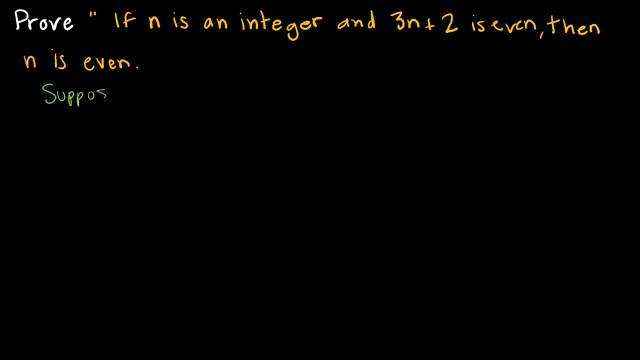 So to start, I'm going to say: Suppose 3n plus 2 is even. However, The original And n is odd. So again, I'm making the wrong assumption at the beginning to be even. We know if we add or subtract an odd number from an even, what do we? 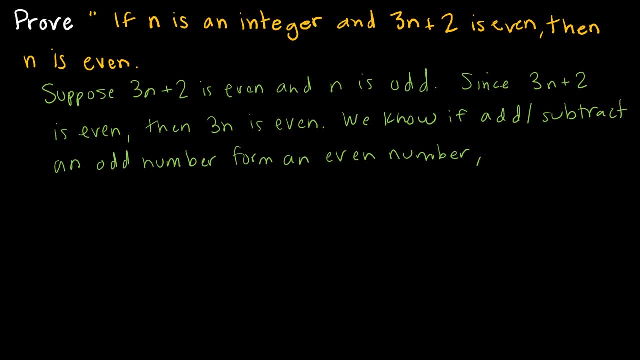 get. If you're not sure, do some of them in your head. So if I take a number like 2 and I subtract an odd number, then I get an odd number. So we know if we add or subtract an odd number from an even number, we get an odd number. So I'm going to take 3n, which 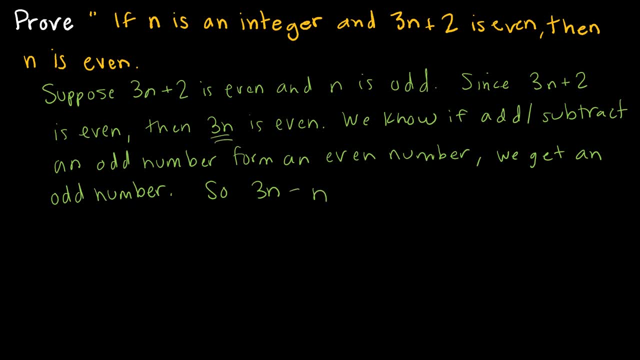 I know is even, and I'm going to subtract n, which I know is odd, and that's going to give me 2n And I'm saying this is odd. Well, why is it odd? Because I just said: if I took 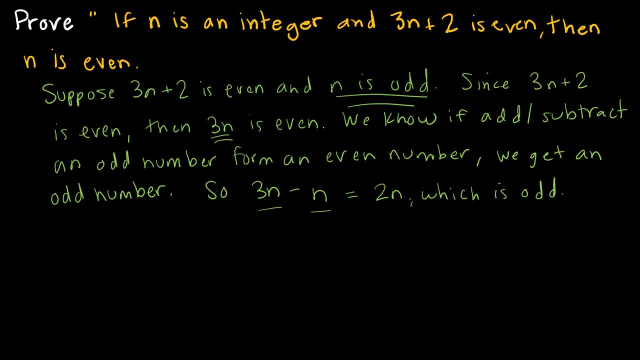 an even number and I subtracted an odd number, I'm going to get an odd number And hopefully you're seeing that this is a contradiction. So, however, 2n cannot be odd because of course it's 2 times some number. So our original statement was false And therefore 3n plus.